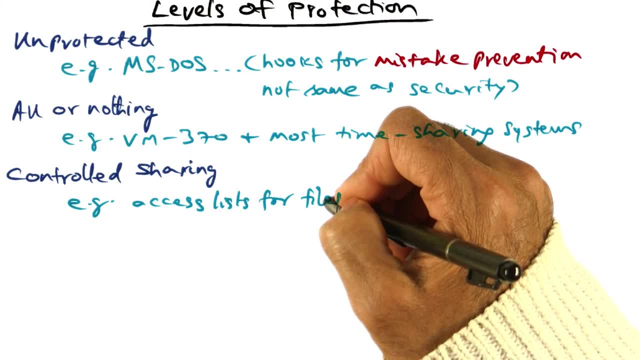 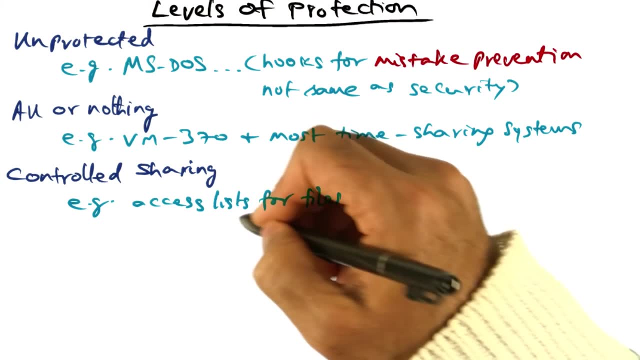 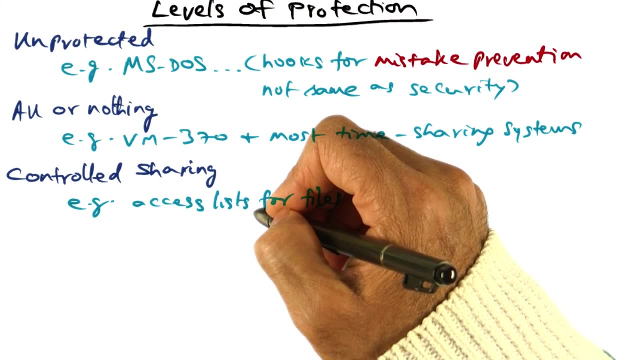 create a file, I could say my file can be shared by my students And here are the names of the students that have access to that file. So that's an access list that you can associate with information that you create and give to the system for safe keeping, That's, controlled sharing And other. 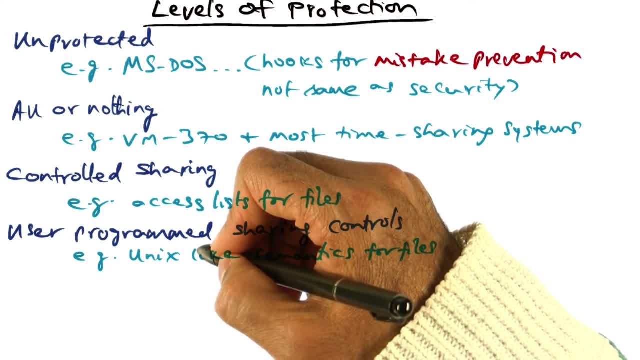 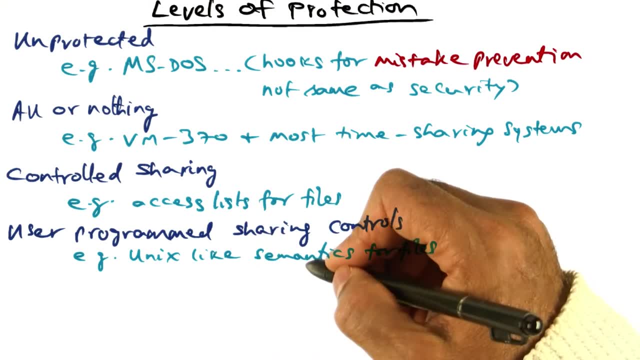 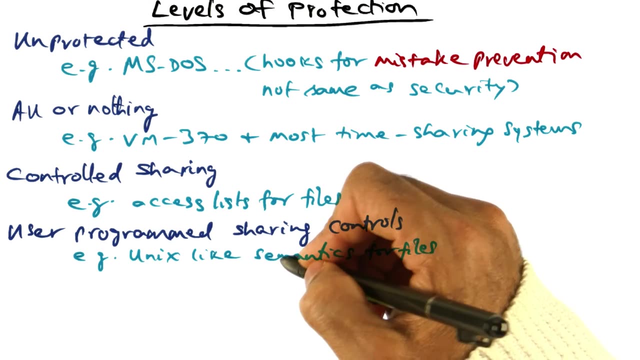 level of protection is controlled sharing, So a the level of protection is what Salsa calls user programmed sharing controls. Now, this would be a facility similar to what you find in Unix file system today, for instance, Such as being able to associate different access rights for. 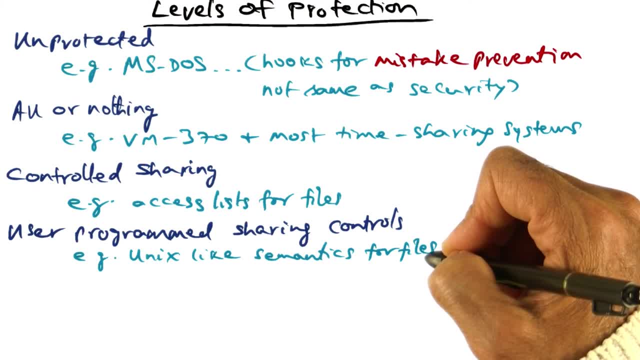 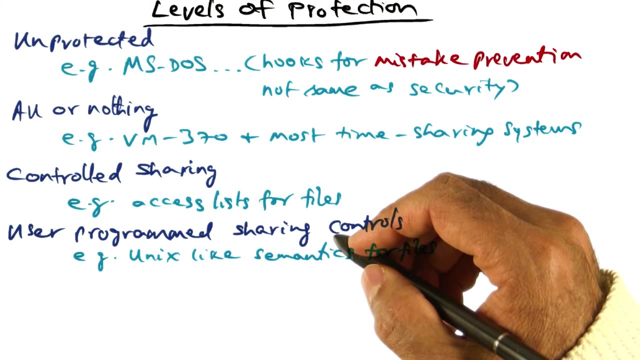 files for different groups of users. In Unix, for instance, there are three levels of protection that you can associate with a particular file that you create. What is the access right for the creator, the owner of the file? What is the access right for a group that is defined? 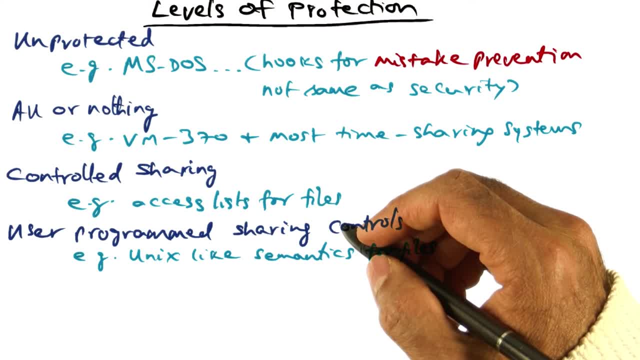 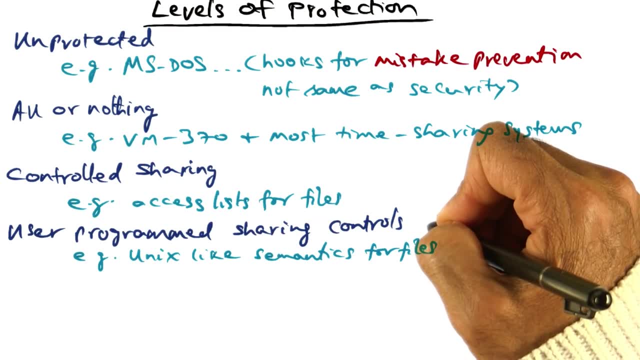 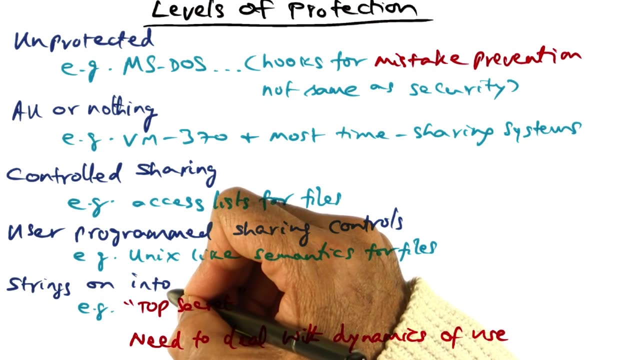 And what is the access right for the rest of the world? So there are three levels of protection that you can associate with a file, And that's an example of user program sharing controls. Another level of protection is having user defined strings on information, For instance in: 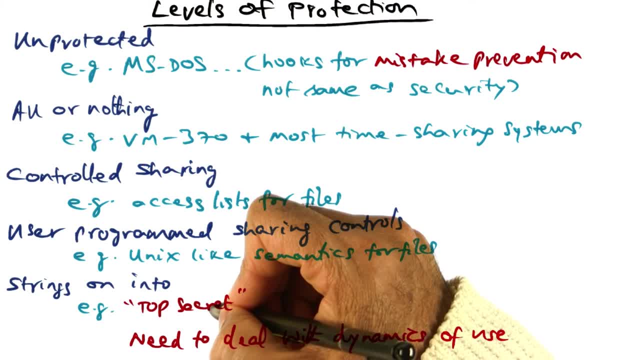 the military, it is often common to have physical files labeled with top secret that has to be opened by only some privileged set of users. Similarly, you can associate such strings on information that you create and store with the system. These four levels of protection that I identified here are not cast in concrete. 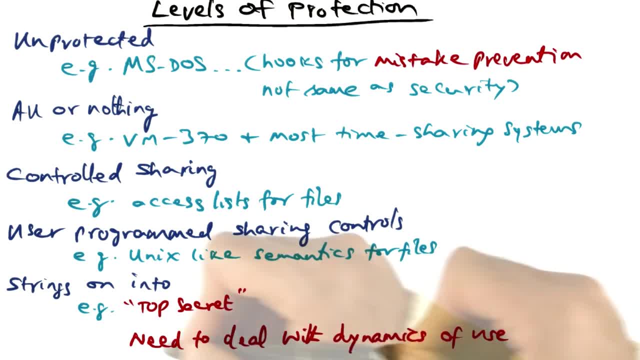 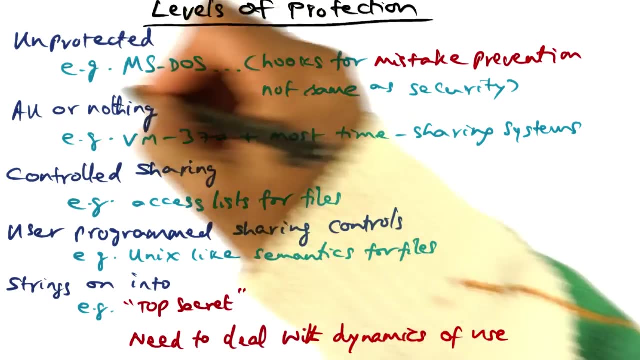 because, as the system evolves, as the user community evolves, you need to be able to deal with the dynamics of use of this information, use of the system. So that is another issue which you can call as a cross cutting issue with respect to these levels of protection. For example, 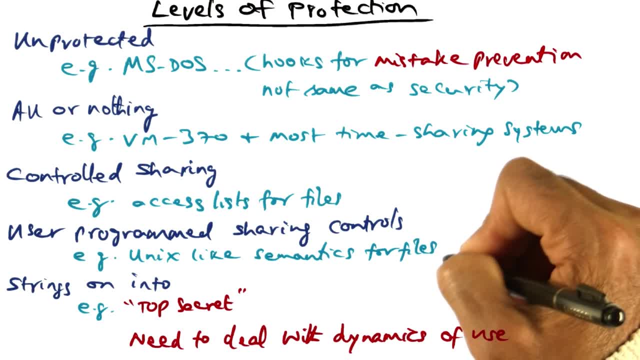 how do I change the permissions I've given to a particular file, to a set of users that I've defined as a group that can access that file? How do I change the set of users I've included in the access list? What do I do to? 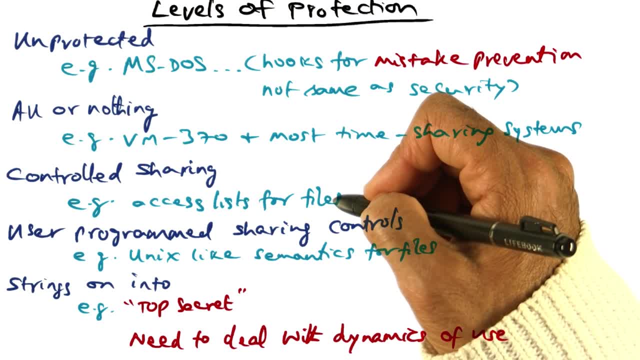 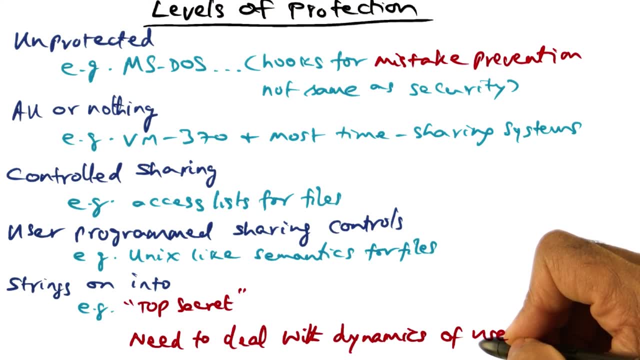 remove somebody from the access list? What do I do to add someone to the access list for information that I've already created? So all of these are issues that deal with the dynamics of use of information.